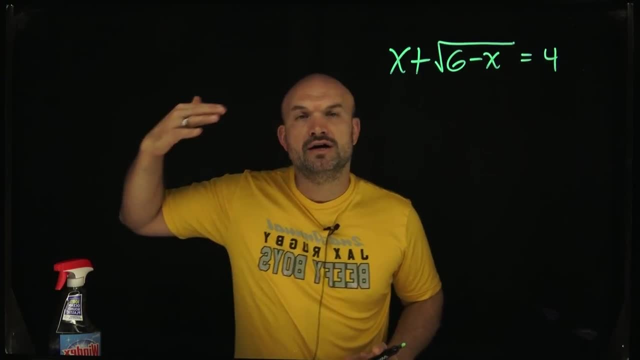 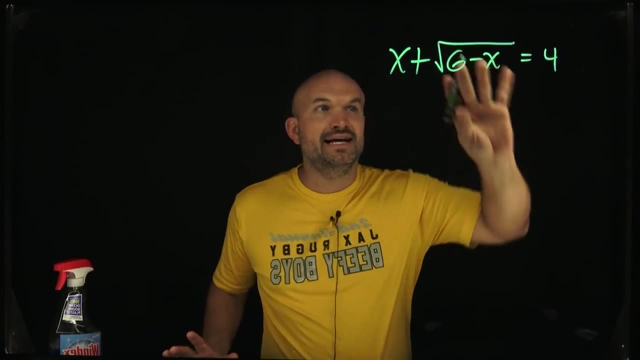 original equation. The main thing you want to do is focus on how do we solve our square root equations or our radical equations. You isolate the radical right, You isolate that square root. So that's the first thing I want you to focus on is getting a square root isolated. That is going. 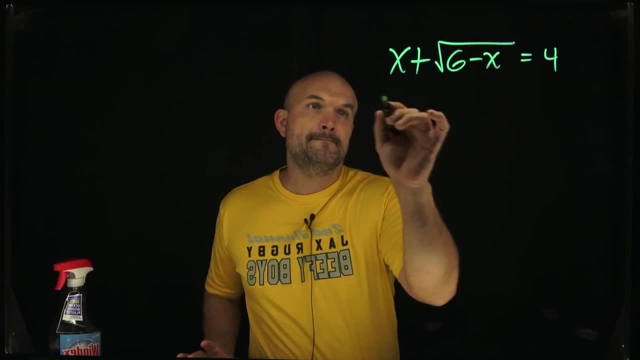 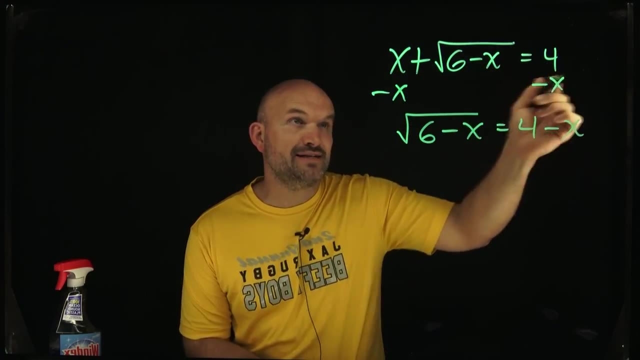 to be what we call, like our original equation, when in an isolated form. Okay, So now what I did is I just, you know, isolated, I just add subtracted, I'm sorry, an X on both sides. So now I have the. 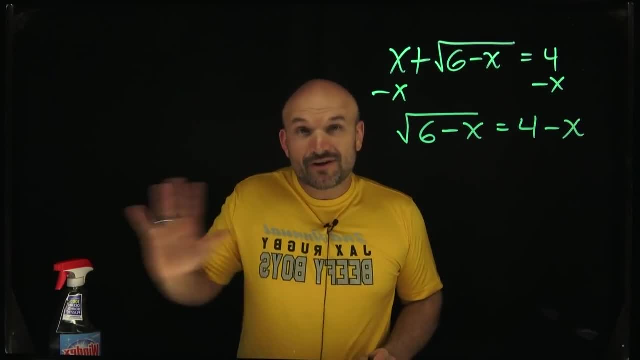 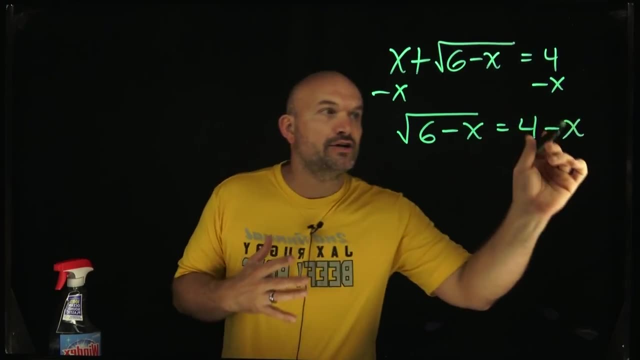 square root to six minus X is equal to a four minus X. Now, if there is going to be extraneous solution, more often than not is going to be when you are squaring both sides, because what happens is right now we have a linear equation, right? So therefore, technically there's one. 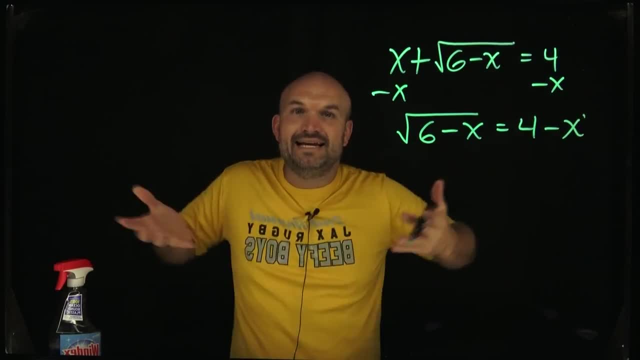 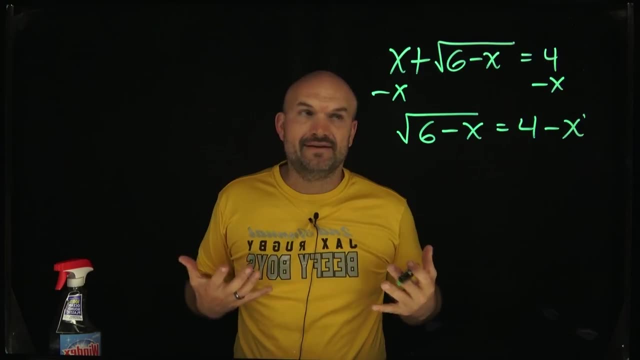 answer. However, when you square both sides, what you're doing is you're creating a quadratic, and remember, quadratics can have zero, one or two solutions, right. So you're opening up different possibilities. And again, the same thing can happen if you're cubing or, you know, raising. 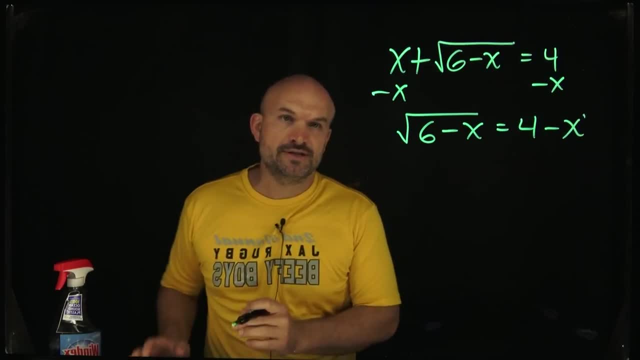 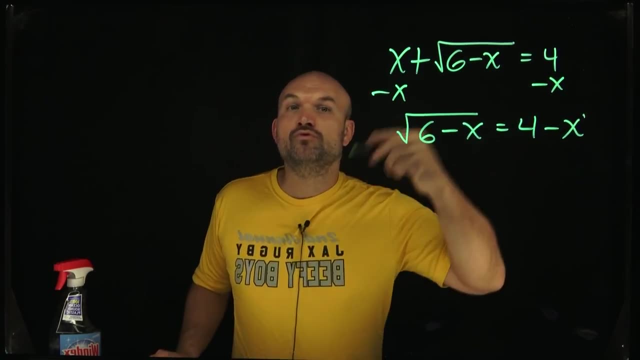 to the fourth power, like you're opening up more options for extraneous solutions. Now, the simple definition for an extraneous solution is a solution that works for a final answer but does not work for the original equation. So this is our original equation. 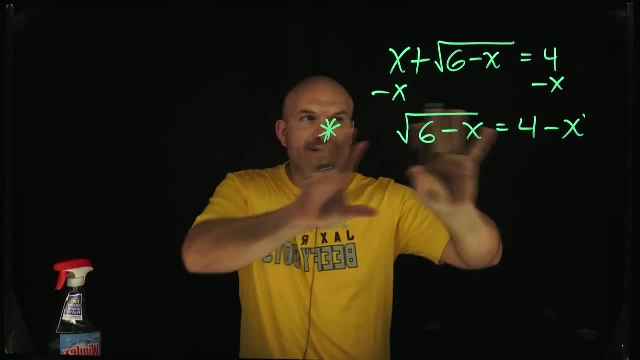 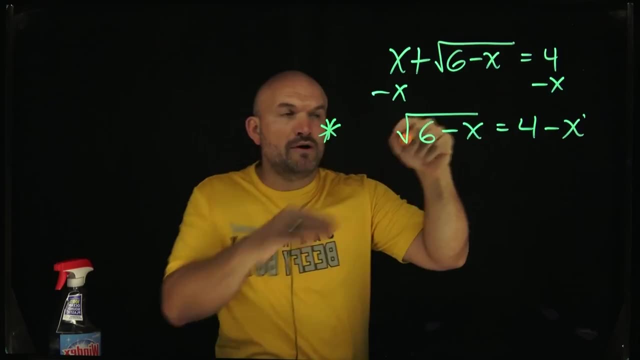 Okay, Just adding the X to the other side is not changing anything, right? This is still our original equation. However, now what I need to do is go ahead and solve this And remember our next step here. when I have a square root equation already isolated, I got to get rid of the square. 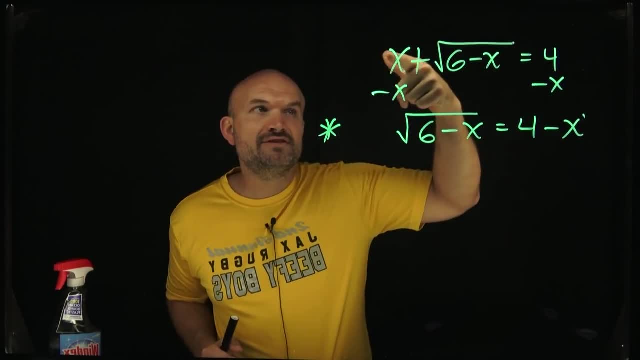 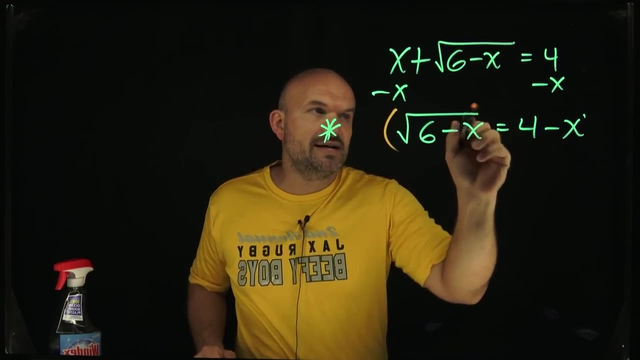 root. So to get rid of the square root, I got to use my inverse operations. The inverse operation of having a positive X was to subtract an X on both sides. Well, the inverse operation of the square root is going to be to square both sides. Okay, So what's important about this is I'm 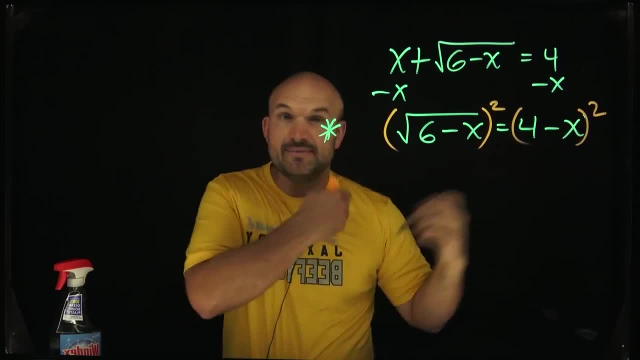 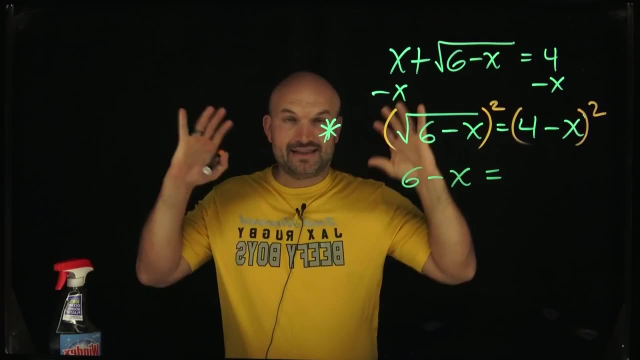 squaring the square root right. So what that's going to do is that's going to eliminate the square root. So therefore, I'll just have a six minus X. But over here, what I want you to see is now: what I've done is I've taken that linear X right And by squaring it I'm now. 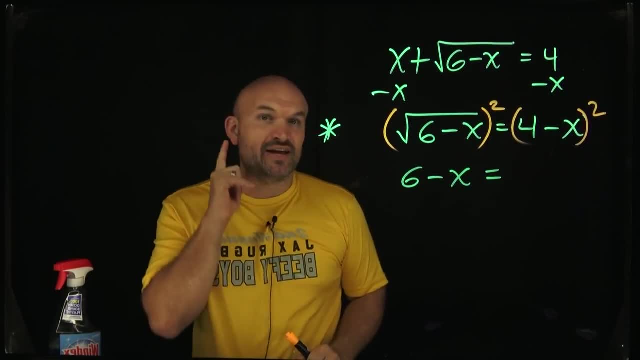 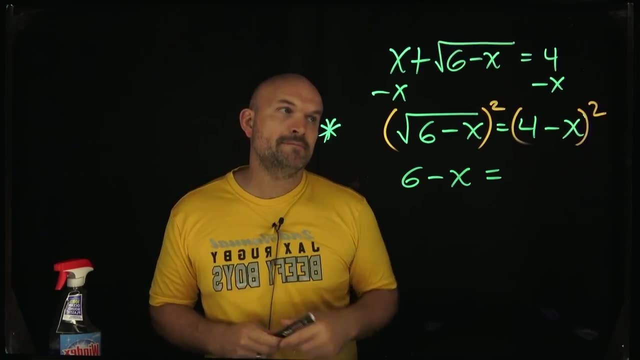 creating a quadratic equation. That should be your point of like. uh-oh, I just created an extra solution. I have to make sure that I look for extraneous solutions. That is critically important, So let's just go ahead and multiply this over to the other side. Do not distribute the two across. 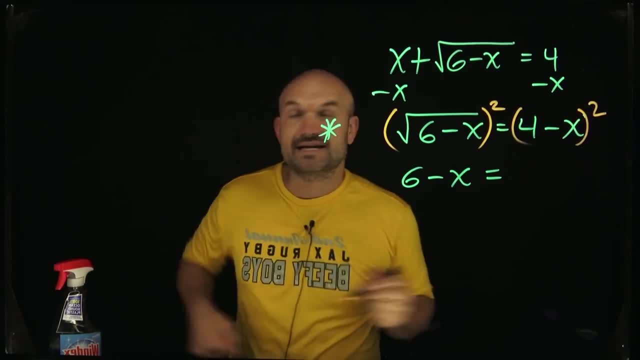 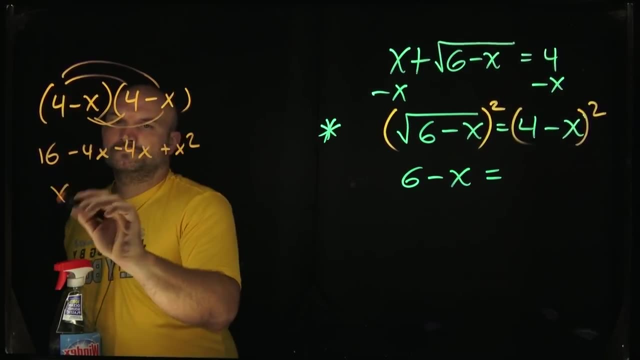 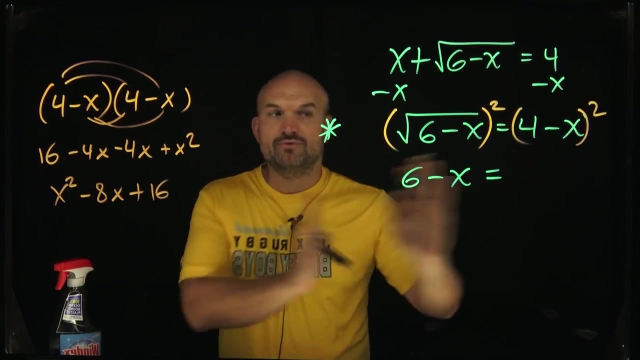 right, Four minus X squared is four minus X times a four minus X. Okay, So I just went ahead and multiplied out and then I just rearranged it So it was a little bit easier for me to kind of read. Um, cause that's exactly how I'm going to write this over here. 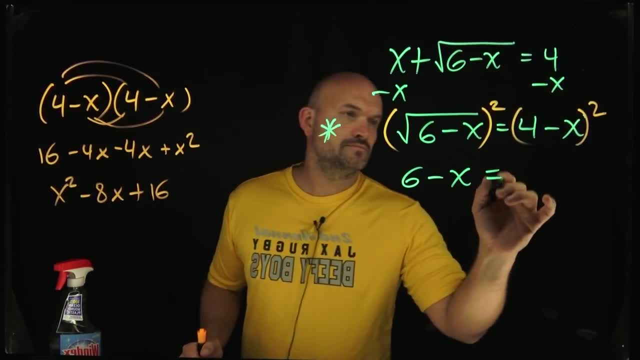 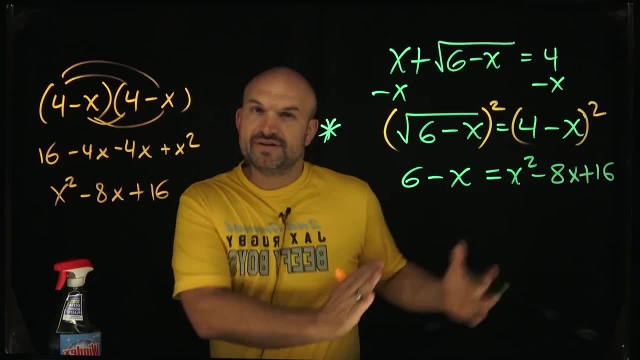 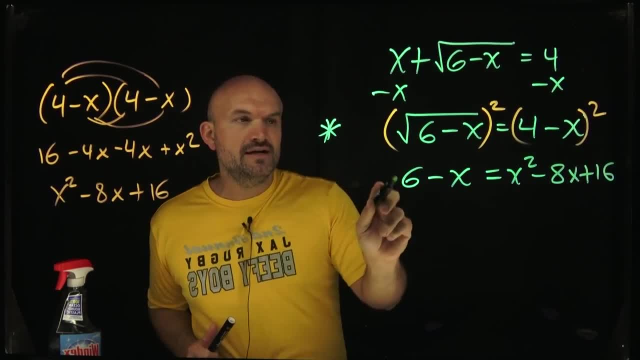 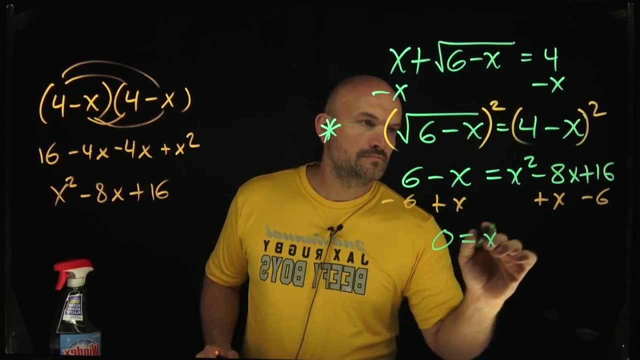 Both sides. here I have a positive six, kind of like had a positive X over here. So to undo the positive six, I'm going to subtract a six on both sides. Okay, So now you can see. um, I have zero. 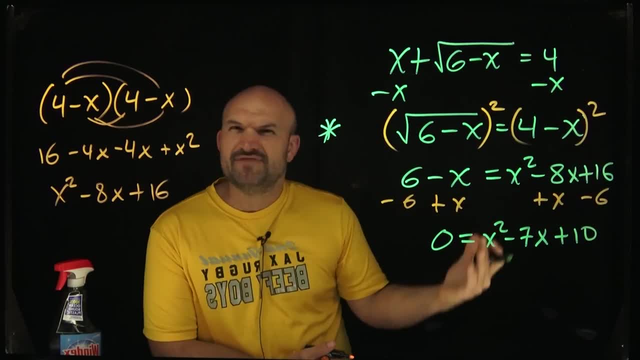 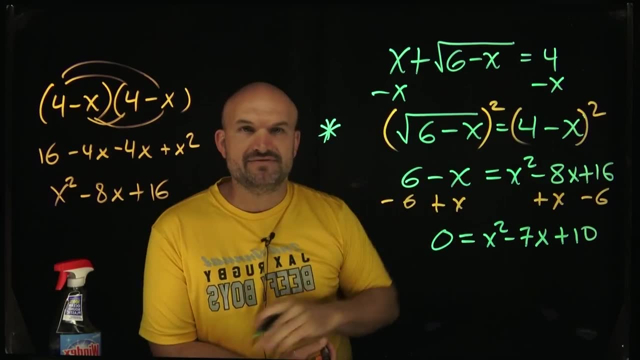 equals X squared minus seven, X plus 10.. Right, And again, like we always want to look to factoring first before you go to quadratic formula or completing the square, And so I'm basically asking myself: is what two numbers multiply- give me 10, add to give me a negative seven. 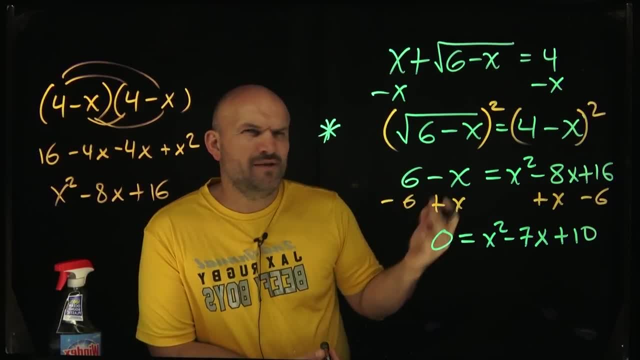 So immediately I'm thinking 10,, well, 10 and one and five and two. right, Oh, 10 and one don't add to seven, but five and two do has to be negative, So it has to be a negative five plus. 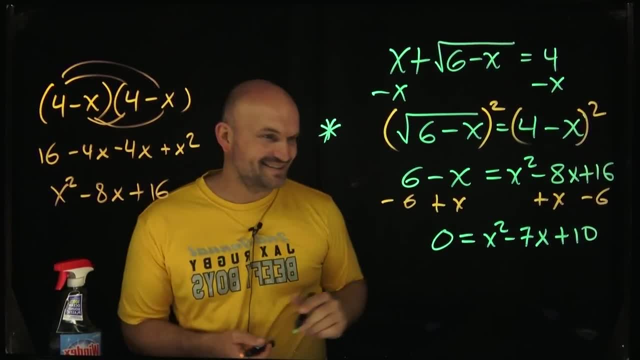 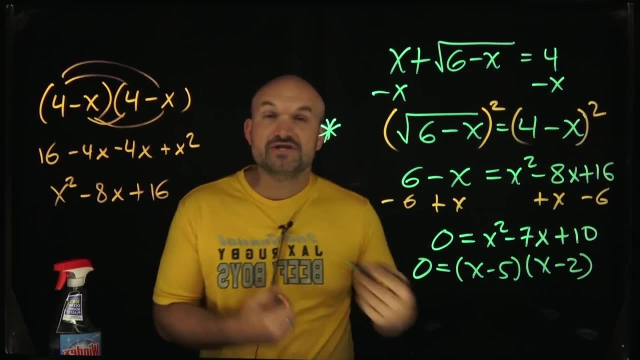 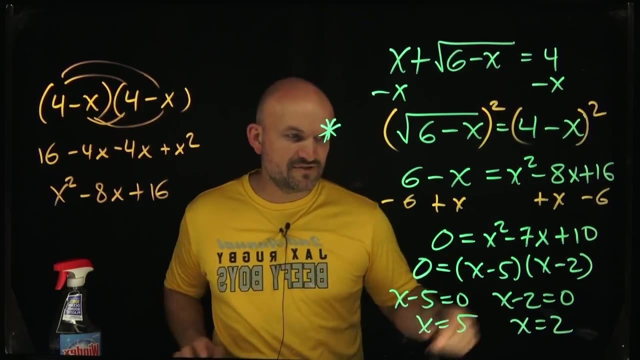 a negative two does negative five times. negative two multiply give me 10.. Hey, Hey, I was looking pretty good. Okay, And remember, now when I have a product equal to zero, I can go ahead and apply the zero product property and then solve to get my two solutions. Okay, So now I have: X equals five. 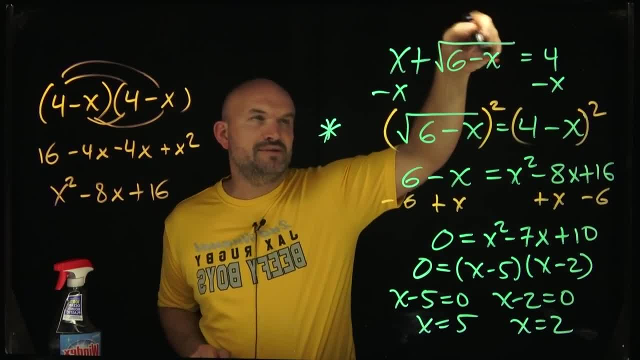 and X is equal to two. So you can plug them into this equation. You can plug them into that equation, It doesn't really matter. but we got to check for extreme solutions, right? Because we went from a negative five to a negative two. So now I have X equals five and X is equal to two. 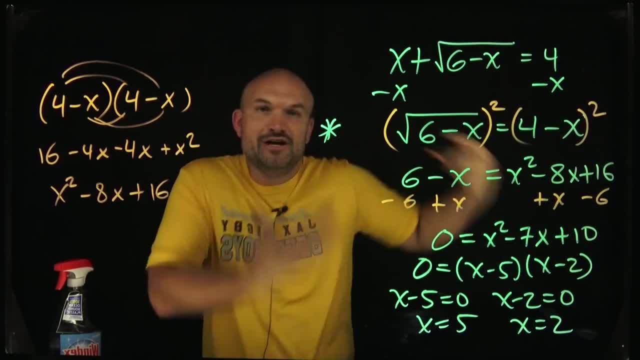 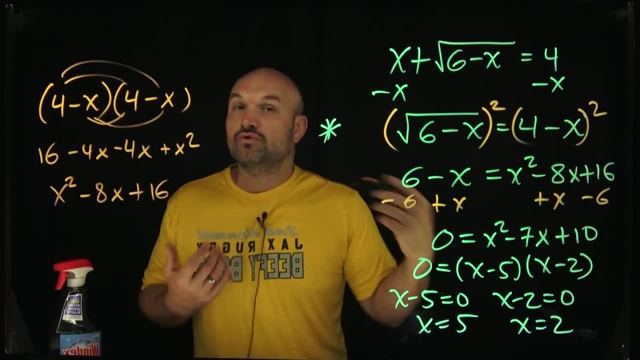 Like a linear, like an equation with a linear X to now squaring that to now a quadratic. So these could both be true, right. And again, the best way to kind of verify that would be to plug it in or look at the graph, right? It kind of depends on what type of math you're doing, but let's just